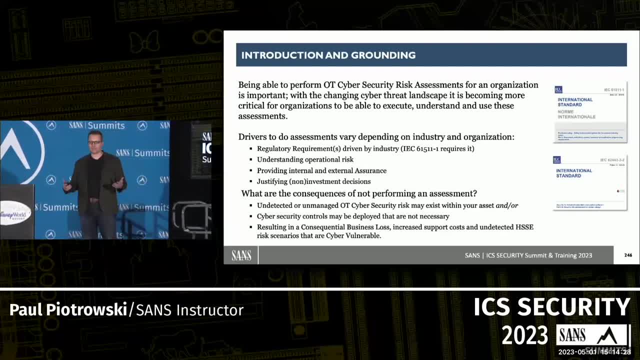 right If you're doing a functional safety project. right? IEC 61511 actually mandates that you do a cybersecurity risk assessment for your safety system, because these safety systems and these new architectures are actually integrated into your BPP-CS right, And so there's. 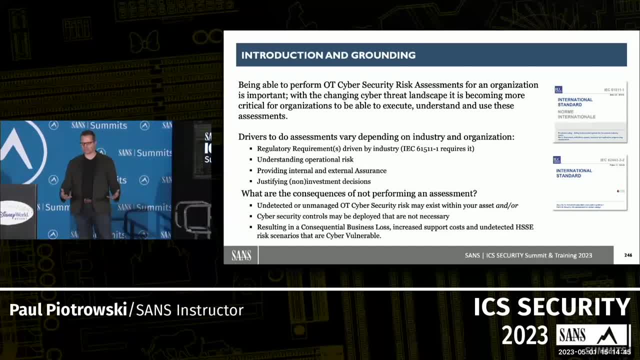 huge risks once you invest in them, And so there's huge risks once you invest in them, And so there's huge risks once you integrate your control and your safety system into one system, right. So that's why 61511 actually mandates you to actually do one Understanding operational risk right, One of 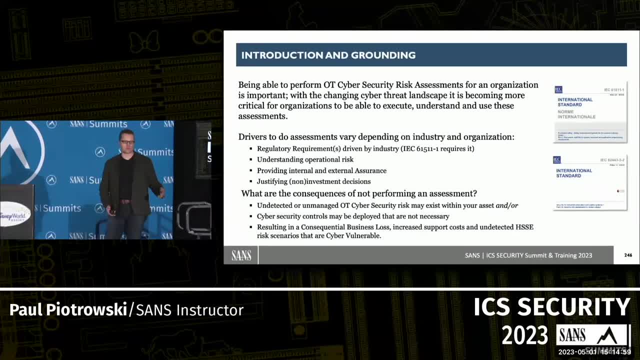 the things that we are trying to move towards is from a compliance-based infrastructure compliance way of doing cybersecurity to risk-based. So you need to understand your operational risk at an LNG terminal at an offshore platform, whatever it might be right, Understanding and owning that. 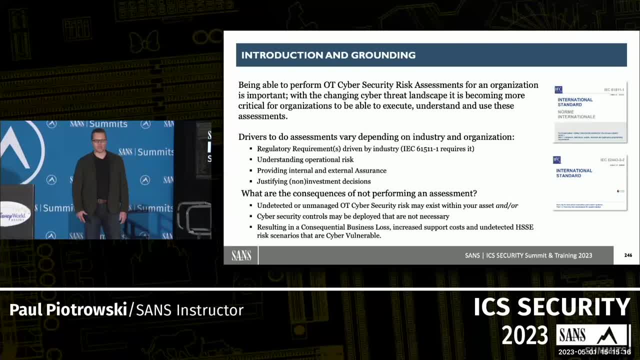 risk is paramount in these complex working environments. We don't have finite, we don't have infinite budgets, right, So you need to restrict, you need to hone in on the crown jewels of your asset, of your line of business, whatever it might be, and put more emphasis on those. 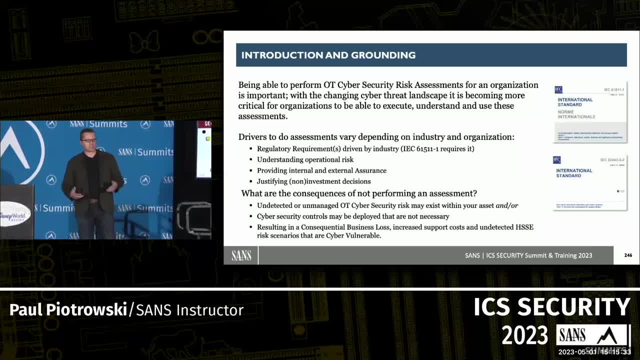 processes or those assets. We actually used cybersecurity risk assessments as part of our internal and external assurance process. Jason, right In the morning he had a presentation about the greater oversight right. We actually use cybersecurity risk assessments as evidence right to our auditors. 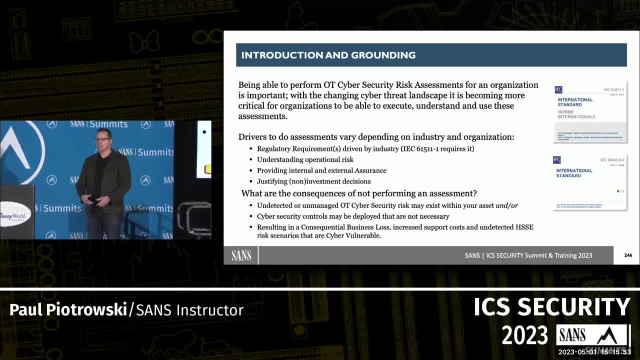 to say: these are the risks, we understand the risks and this is what we're doing right. So it's almost like evidence-based right To say this is why we're doing it, because we did a cybersecurity risk assessment and this is the output of it, And also for justifying investment. 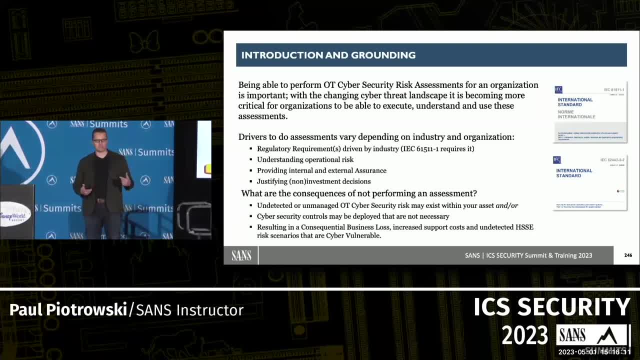 and non-investment, So we need to understand the risks right, And also for justifying investment: investment and non-investment- So we need to understand the risks right- And also for justifying investment decisions. One of the cool things that we actually did just recently: we did a safety. 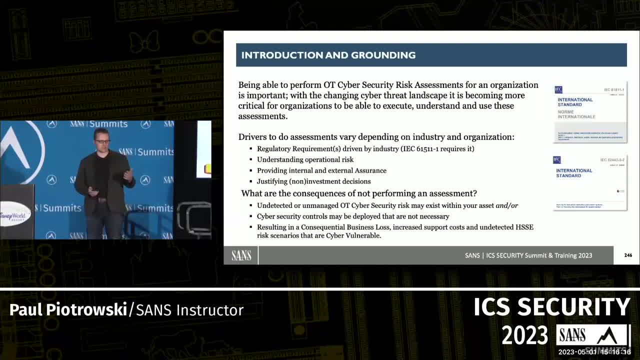 risk assessment and we determined that one of the zones that we were assessing was low risk and there was no cybersecurity risks associated with it, And the sparing philosophy for the outdated equipment was sound and the vendor still had actually had the equipment, But in the capital. 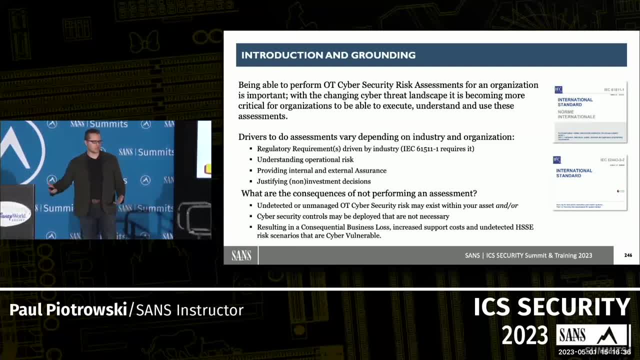 investment plan. the asset wanted to spend a few million dollars actually upgrading right that equipment And we said: hold up, hold up. The cybersecurity risk assessment is deeming it to be low risk. your sparing philosophy is robust and your vendor still has the equipment. Don't spend that money. 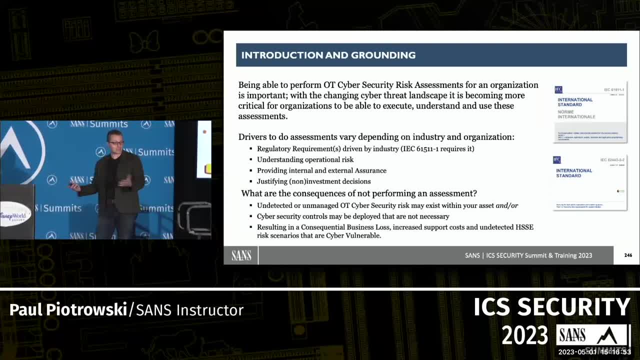 doing that upgrade, spend it over here. So that's actually a very unique case where that cybersecurity risk assessment helps in that capacity. So what are the consequences of not doing a proper or performing a cybersecurity risk assessment? You actually might be implementing too many controls in your organization and you're not doing a proper or performing a cybersecurity risk. 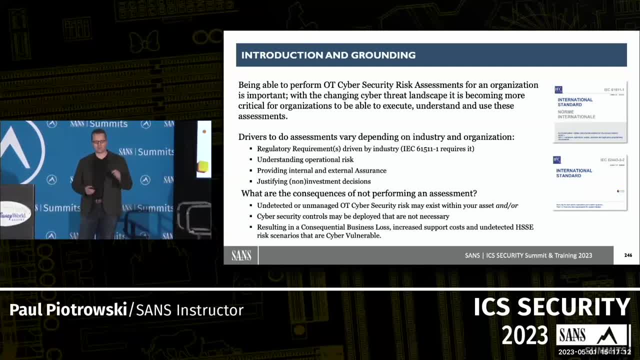 assessment which is going to cost you money, right? You want to fine tune the controls and put the real emphasis on your critical processes, And then the kind of the holy grail of what you want to obtain from a cybersecurity risk assessment is: you want to determine, at the end of the day, 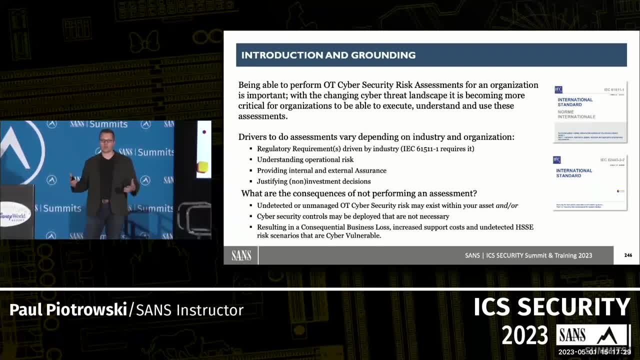 if any of your threat lines are actually fully cyber hackable, right. Ideally for your real critical processes, you want mechanical, non-hackable controls to keep your plants, your asset, your production, operational. This is a bit of an evolved kind of topic, right, And we 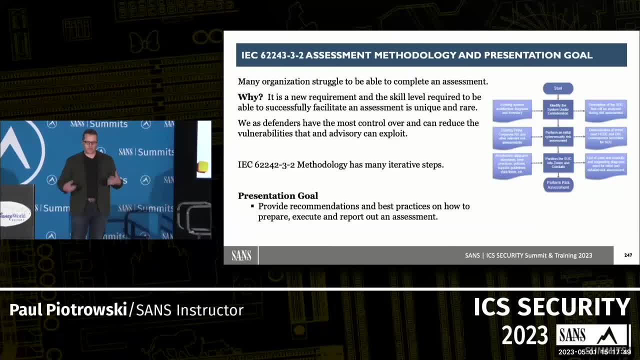 can cover it right if we have time. So I'm not going to be going through the intricate processes of the 6243 standard right. I want to kind of get into the more meat and potatoes of the learnings that we have obtained from the work that I've done for the last two and a half years. 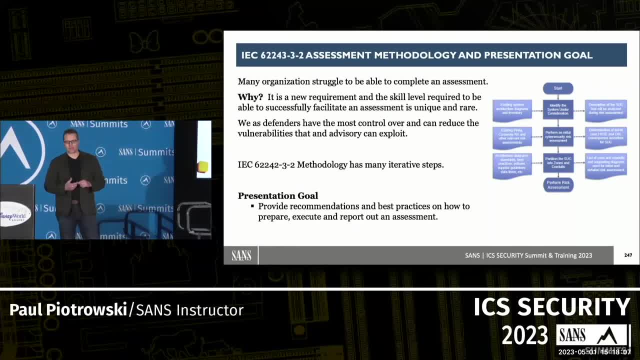 I think that's a lot more value add. You can download this standard. it's not free right like the NIST framework right. You have to pay around $200, $250.. Last time I downloaded it for one copy- or you can buy an enterprise license from the IEC and get documentation. 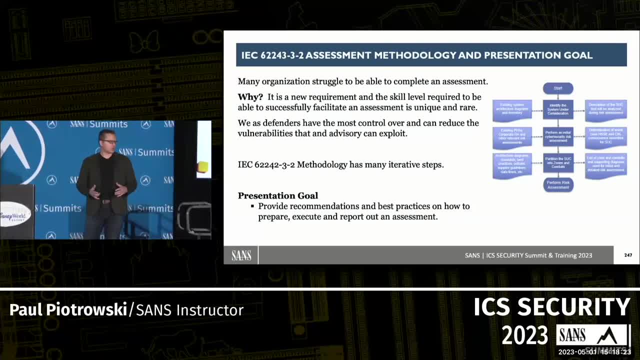 But one of the first steps that you need to do is you need to demark what you're actually assessing, right? They call it the SUC system under consideration. So you really have to draw a line of what you're assessing, because you don't want scope creep right in your cybersecurity. 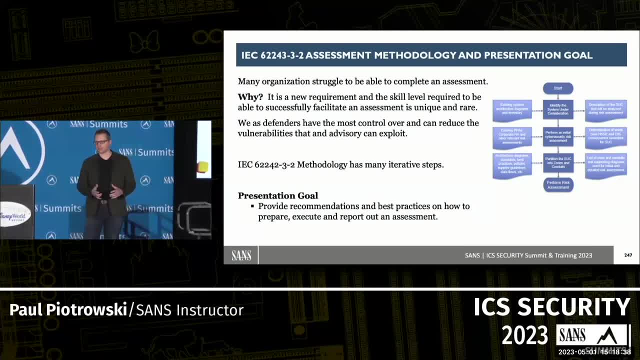 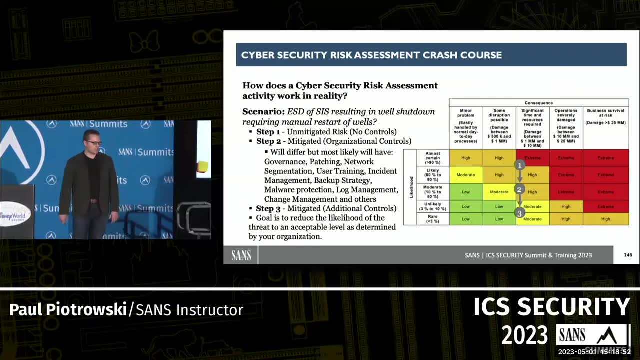 assessment And then, once you decide what your system under consideration is, then you have to break up the network into zones or functional zones, and then you go through different threat scenarios and evaluate the risk. So one page crash course for anybody that hasn't actually done. 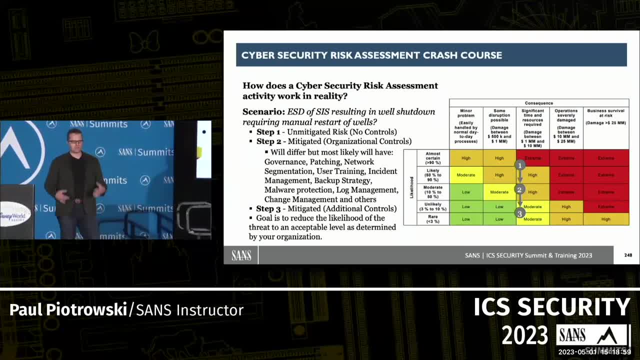 a cybersecurity risk assessment. The process is: you basically start with an unmitigated scenario. So you talk about a particular scenario over here. It's an emergency shutdown of some wells in the field, right, that requires manual restart, So a guy would have to get into his truck and drive around. There's exposure hours associated with it. 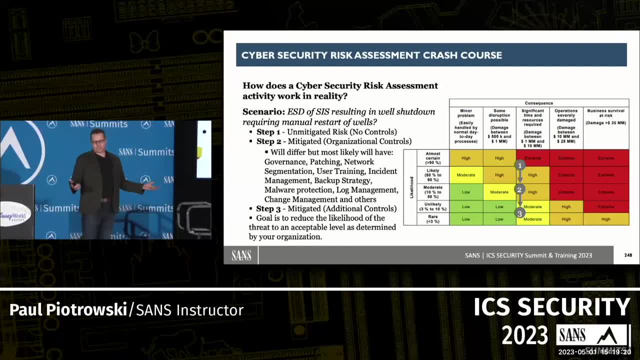 to reset the wells right. This is obviously going to cost money because the wells are down right. So you'd say, okay, that's going to one day of outage is going to cost me $3 million, or whatever it might be right, depending on your field. Then you say, okay, that's unmitigated. 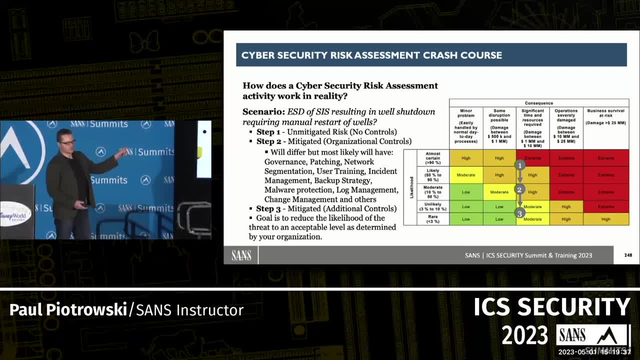 and you mark, You know, on a dot on your matrix, on your risk assessment matrix, And you select a square. Then you say, okay, what controls do I have? Well, I have physical security. I have defensible architecture. Maybe I did a wicked tabletop right that Mike facilitated last week. So my 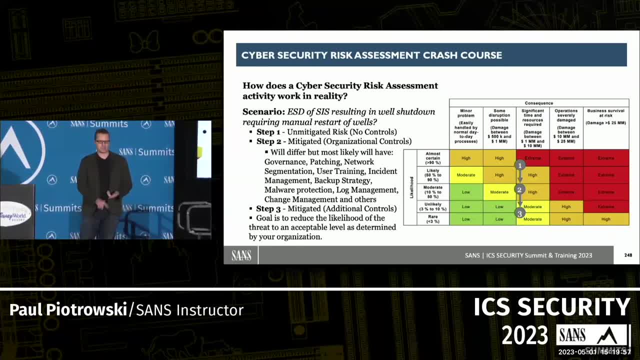 incident management process is sound. You know, I do access controls, I do some system hardening, all that kind of stuff. Then as a group, right in the the workshop, you say, okay, that is going to reduce the likelihood to a certain amount, Bumps you. 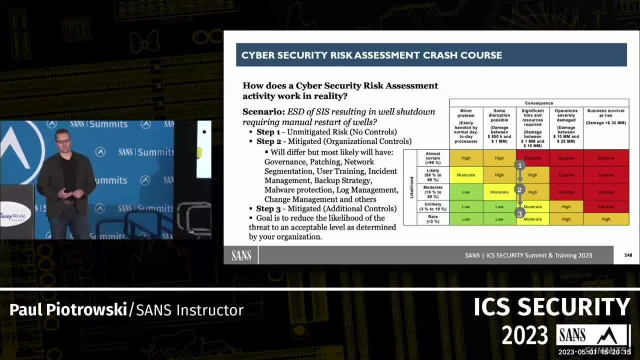 down to another spot, reducing the likelihood. And then you say, well, there's maybe some additional controls that we might implement and it's going to reduce the likelihood even more. The consequence doesn't change, just you're reducing the likelihood of that materializing. All right. so tip number. 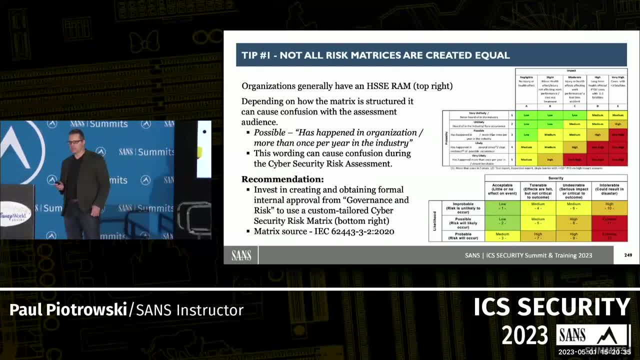 one. all matrices are not created equally Right. So when you go to an organization, a mature organization, they will most likely have a risk assessment matrix that goes into the HSSC or pair right. people, environment, asset, reputation. 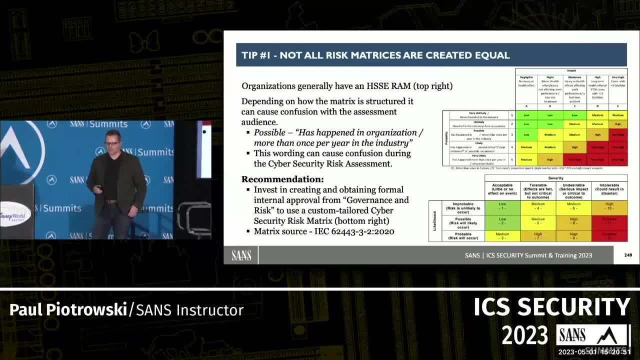 right and they kind of risk. they have identified what is acceptable in the organization and red is bad, you know. green is acceptable and you know and the sort. So this does not work very well for a cybersecurity risk assessment because the HSSC. 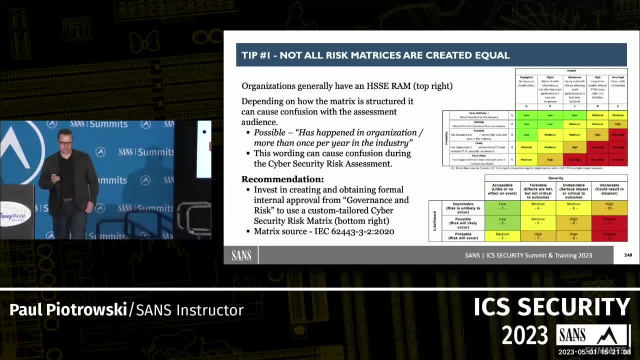 RAM matrix doesn't take into consideration sabotage and it doesn't work very well for an iterative process. So IEC 62443 3-2 says: invest in creating a specific matrix. it can be very similar to the HSSC one, but it has to be cyber specific right and you have to associate probabilities. 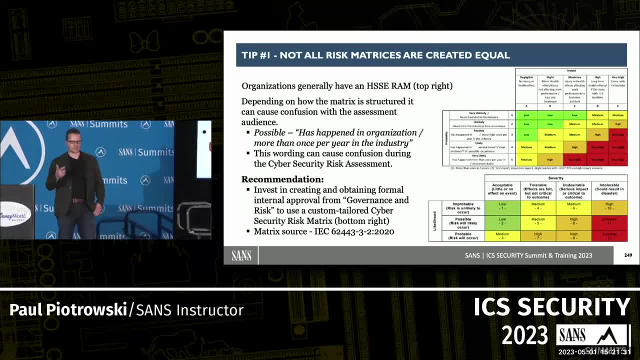 there right, whether it's likely to happen or very unlikely, and you can be a three by three, four by four, five by five. I wouldn't say go, You know a five by five matrix, it becomes too granular, but four by four, five by five is kind. 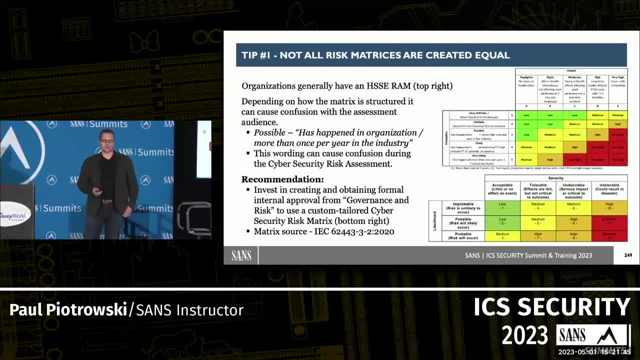 of perfect. right, This is a lot. you have a front load. right. this activity: right, This is not something that you just you know, whip out on a Friday afternoon. right, You have to get necessary people involved. right, Governance and your risk teams have to approve it. it has to be communicated. 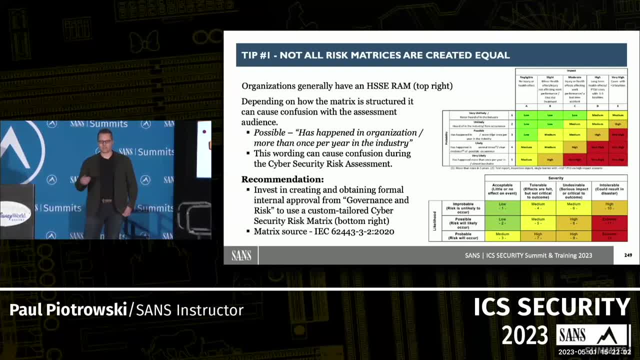 lots of documentation on the justifications of it, etc. etc. But this makes it much easier to facilitate when you go into a workshop because, depending on the language right In the in the HSSC one, it can generate a lot of confusion with your operators and your functional safety. 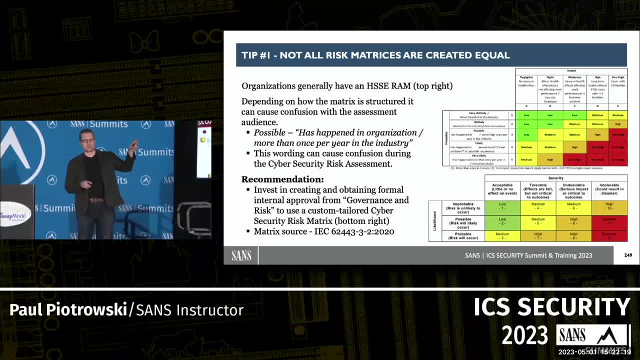 staff to say: well, it says this, it says it should happen in our organization, right, You know for possible or something like that, right? And then it just, you just go off off the rails, right? So you really want to be tactical, right in the questions and and make sure that everything. 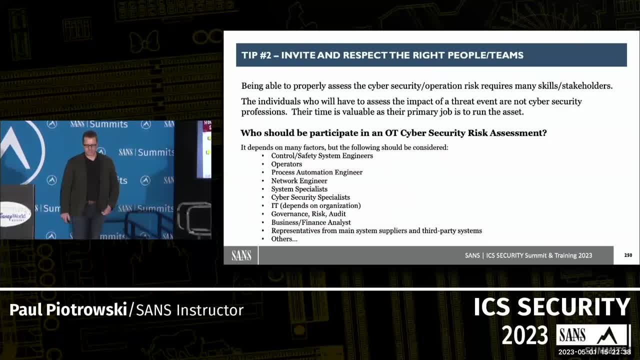 is nice and tight when you do these risk assessments. Who should you invite right to these risk assessments? It should the more people, the better, that know the process, that know the asset. You want to talk to the engineer who knows right what happens right to this. 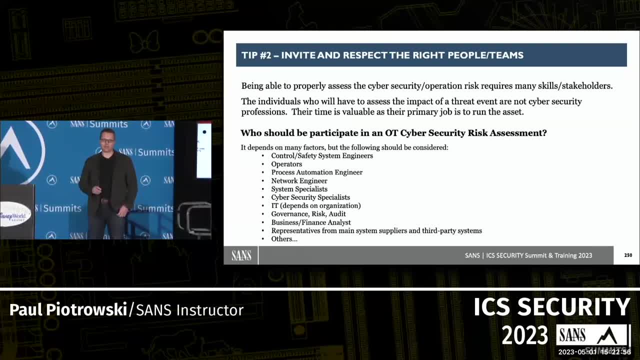 vessel if it's over pressurized. What happens if this valve shuts- shuts right Or the drain header closes right? What is the impact? Is that going to be over pressurization? Is something going to explode, right? 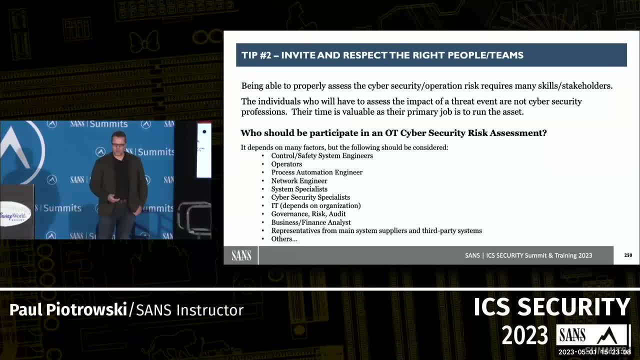 They need to understand the process. So you need operational people, you need functional safety people, you need maintenance- right, There's a lot of people that need to be involved. You also need finance people, because you're going to get into discussions on what happens to my asset if 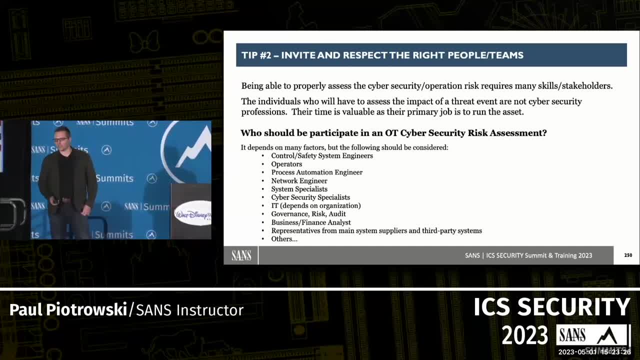 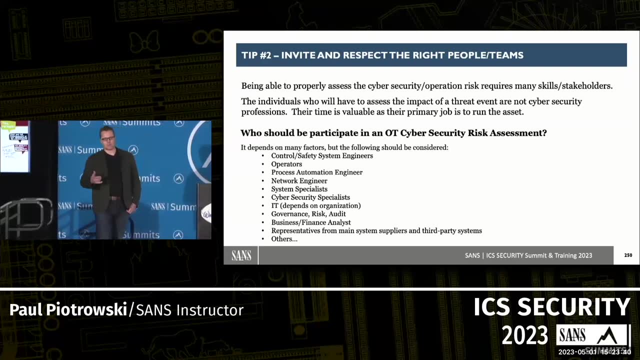 I lose one or two days or or or a whole month of production, right, The finance people need to know that one you know one day down is going to cost you $3 million or $100,000, or whatever right. So you need to have that insight and you have to have those. we call it consequential business loss: right, A lot of these cyber attacks, you know, are not going to be taking down your safety system yet, right, But it's mostly ransomware. Oh shit, you know, we need to. you know, rebuild a machine? right, It's going to cost us this much time. right, We have to buy some. 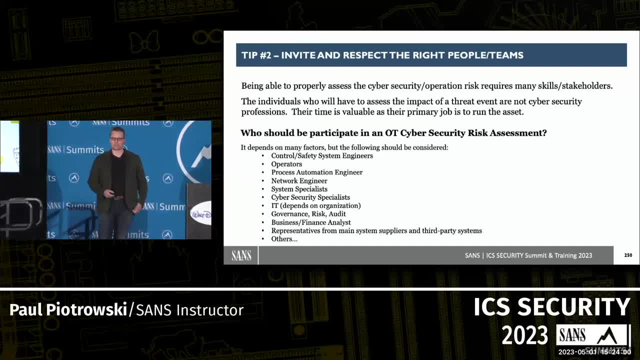 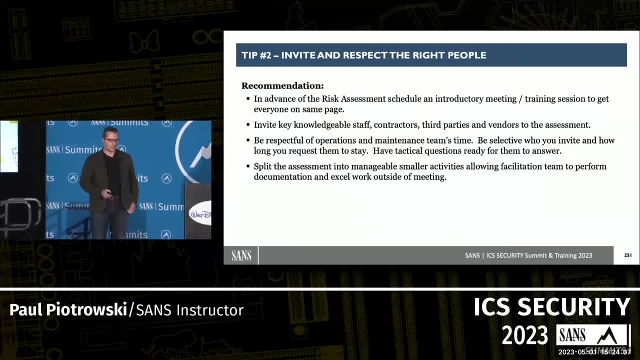 new hardware or whatever it might be right. So those are kinds of the situations that you need, that you have to have those numbers in hand when you're doing these cyber attacks, Security risk assessments. So respect people's time. Operations is very busy, So I don't like. 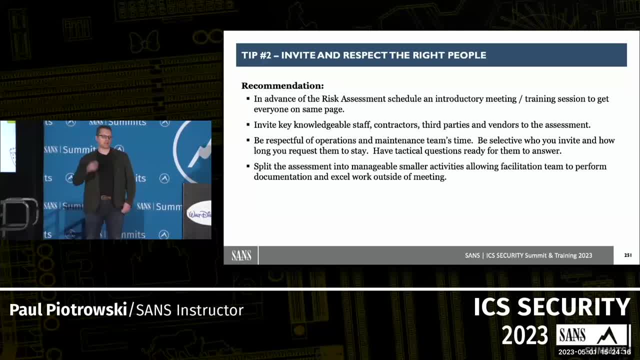 booking full day workshops. when I'm at an asset, I like to have very tailored discussions to say, this day we're going to book an hour or two hours and we're going to be talking about your engineering work zones, or we're going to be talking about your historians or whatever it. 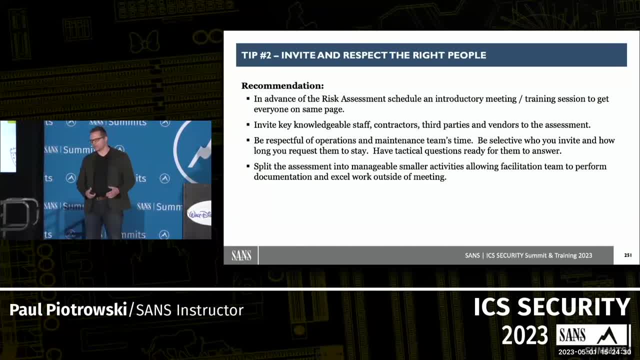 might be. So people come into that workshop and they know Paul's facilitating- he's going to be talking about the engineering work zones or the wireless tablets or whatever zone we pick- And they come in that. and then I have very, very poignant questions for 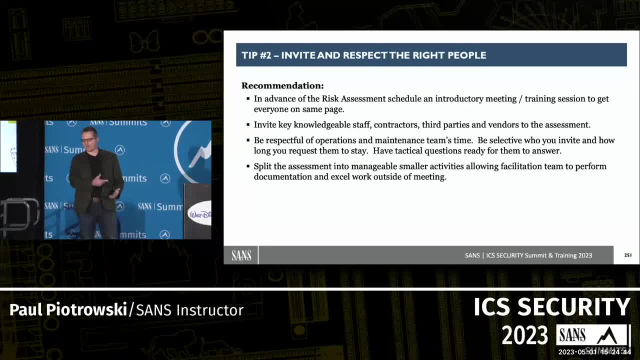 them, And then everybody, we get the results right, That we map it back to the risk assessment matrix And then people go on. they're able to go out into the field, keep operations going. The following day we have another meeting for an hour or two to discuss another zone. 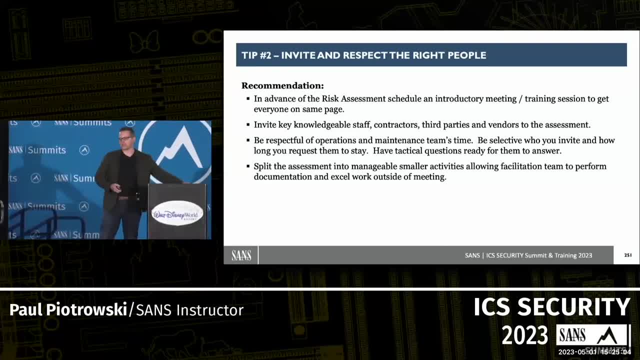 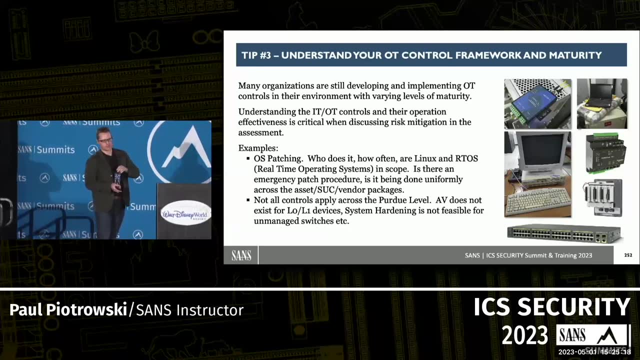 Invite your vendors right. Sometimes vendors and third parties integrators actually know the system better than you, So make sure that you invite the necessary people that are knowledgeable on your system. Understand your OT control framework and the maturity Very key. You don't want to be going into a workshop and not knowing how many media. 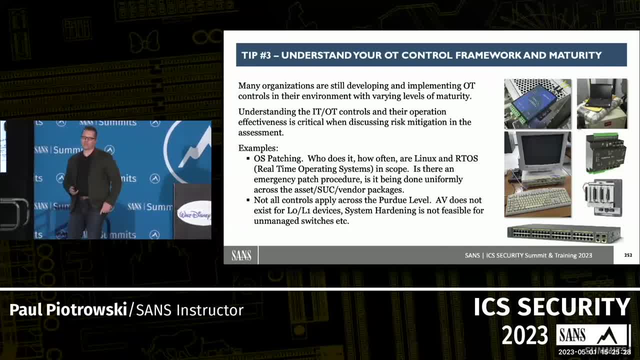 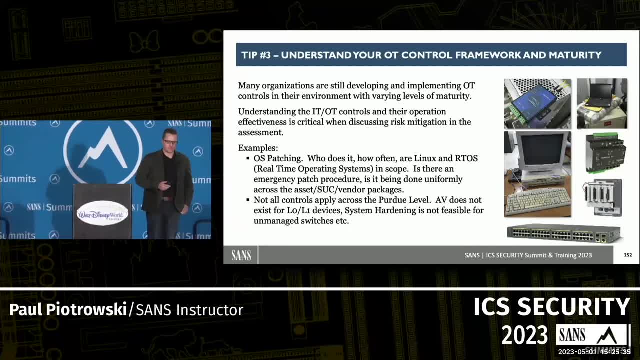 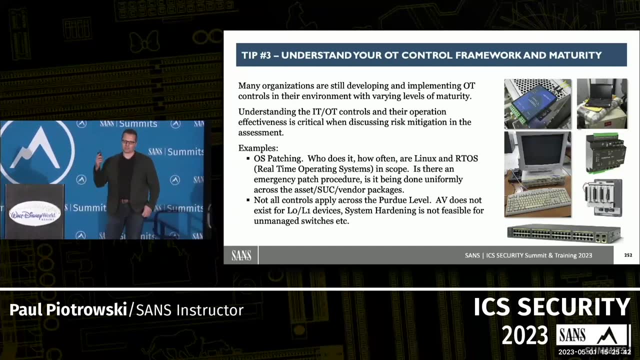 gateways or how many HMIs you have right, Makes it very difficult for you to assess and talk about the zone Knowledgably right If you don't know how many devices you have right. So understand how many technical laptops you have. Understand how many virtualized servers you have. Do you have any old? 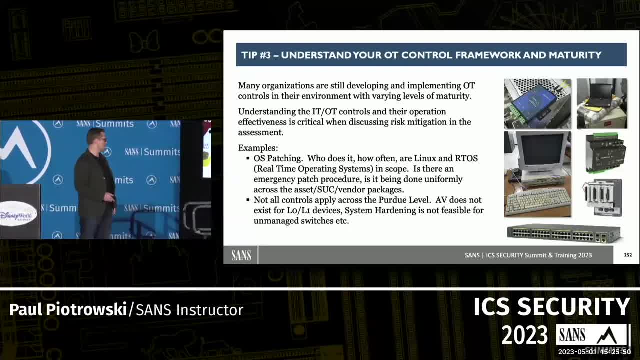 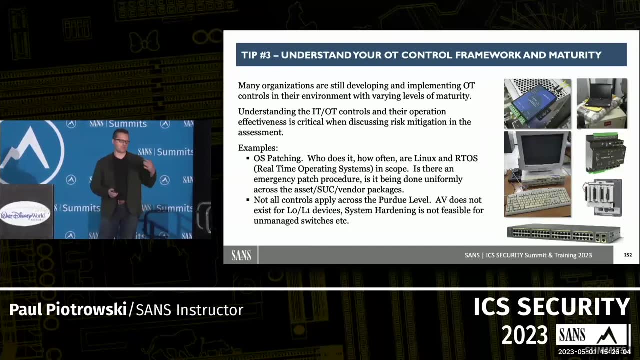 Solaris boxes, right, Linux- you know the list goes on. And then also understand the maturity right. I've gone into a lot of different risk assessments, where you sit around a table or in a Microsoft Teams session and you start talking about patching or network configuration firewall. 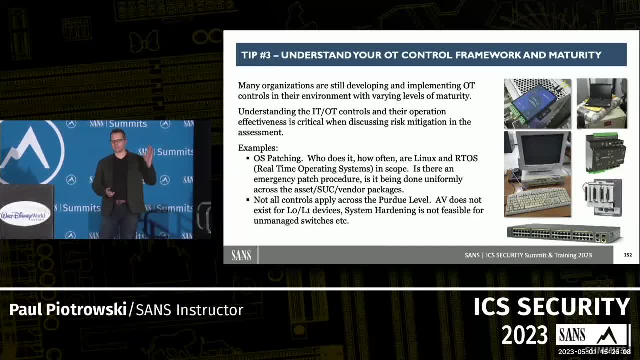 protocols etc. And somebody says, yeah, you know, we have GPOs, you know, installed right, It's all you know, system hardened. And then somebody else pipes up and says, oh no, you know that's. 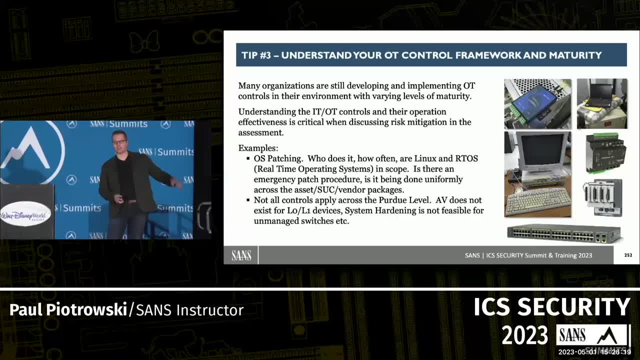 actually this network here is not actually connected to the domain. We haven't done that yet. Or this vendor had a problem with AV. it blue screened right. So AV is not fully operational on this host, you know. and then you start getting disagreements right in the workshop. 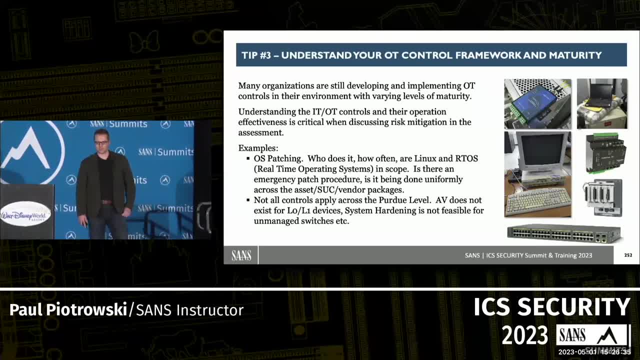 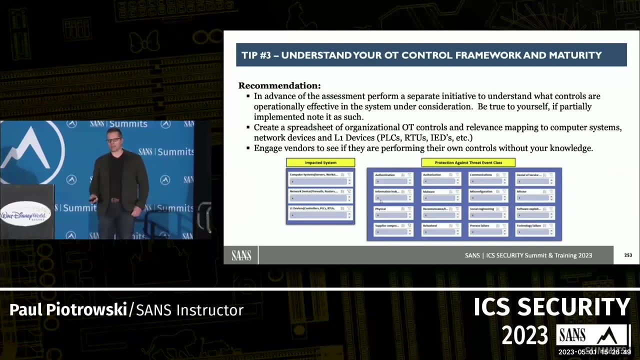 And so that's very counterproductive. right to an organization. And you have to understand the control framework with respect to different controls across different zones. right, So certain zones don't have applicable controls. So if you have an unmanaged switch- right, you know your AV controls are you right, You can't system. 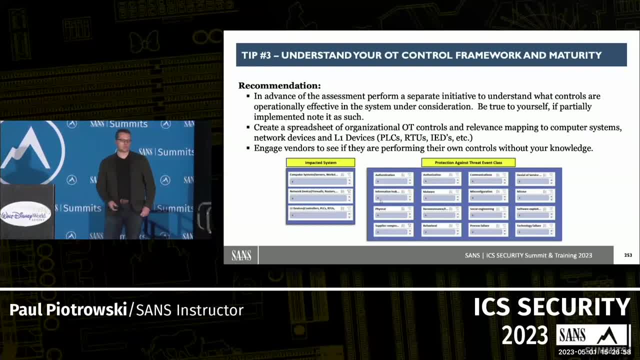 harden an unmanaged switch right, A PLC right? You can't, you know, do an OS patch. So what we've actually created at Shell is almost like a spreadsheet where we have all our controls listed And the asset actually answers which controls. 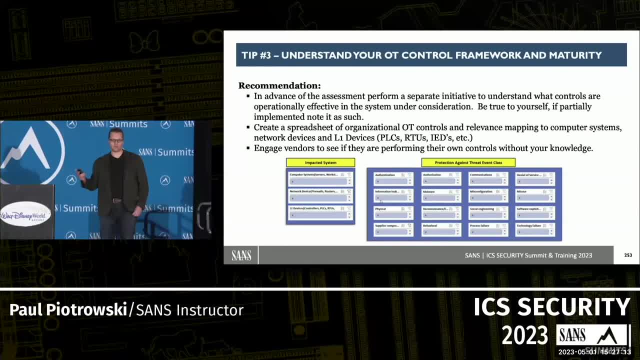 they're actually doing. And then we map them to different components in our OT network, whether it's a PLC level 0,, 1,, 2, 3 device, right? So when we're talking knowledgeably about what controls can we implement? right, we have mandatory controls, optional controls And, within the 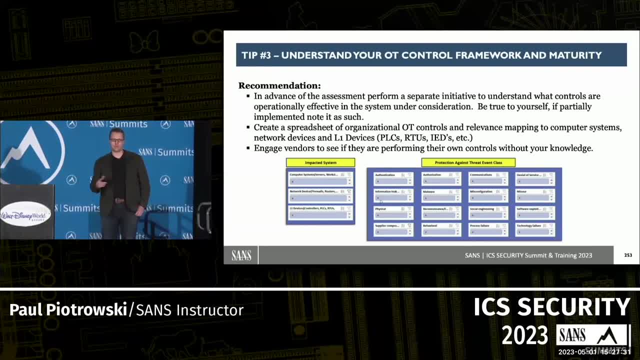 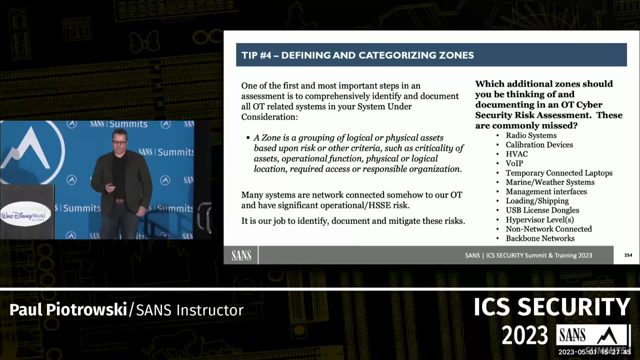 spreadsheet right. we can quickly search. right, what are you doing, What is applicable to a PLC And what controls can we implement. So it makes control selection and inputting it into the spreadsheet that much easier. All right. defining and categorizing zones: right. So this is a big one here. right, There's a lot of. 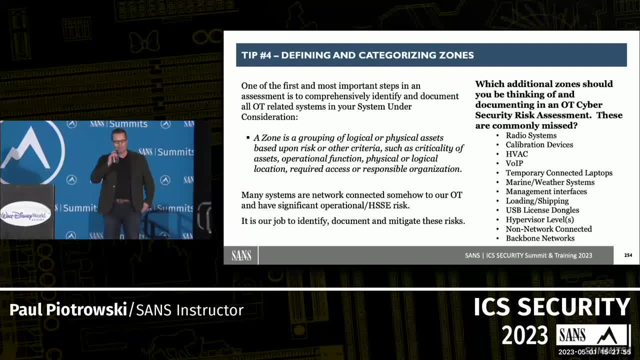 zones that I feel that are missed, that we've actually kind of identified, that I want to share with you. So the definition of a zone is a grouping right of logical or physical assets based upon risk or other criteria. So when you do a cybersecurity, risk assessments obviously. 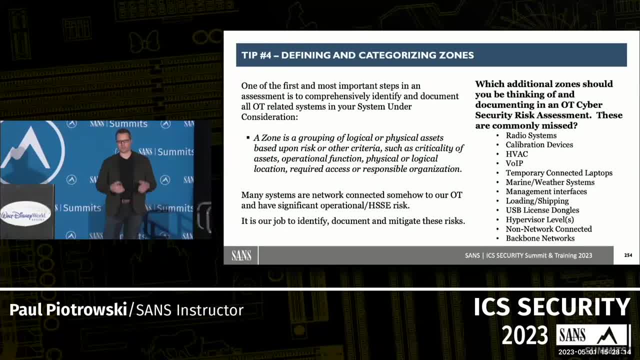 you want to look at the network diagrams. you want to do a go see, you want to look at. you know, open up racks, the front and the back, you know, get a nice inventory of all the systems, et cetera. 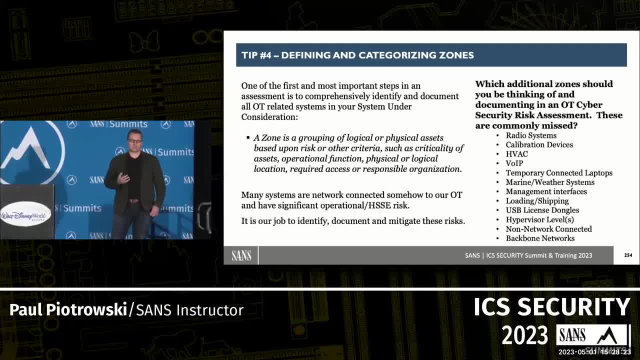 But a lot of the times there's a lot of things that serve a critical purpose in our assets that are not listed on the traditional OT kind of asset inventory lists, for example the HVAC system right. So of course the HVAC system is usually not under the direct system under consideration. 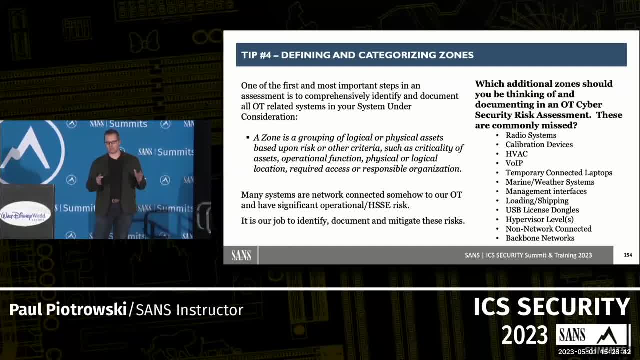 but when you're working at a chemical plant or a refinery, the HVAC system in the building and in the control room is usually critical because it pressurizes it right from explosions and from gases Right. So we've found certain situations are not obviously not directly connected into our OT. 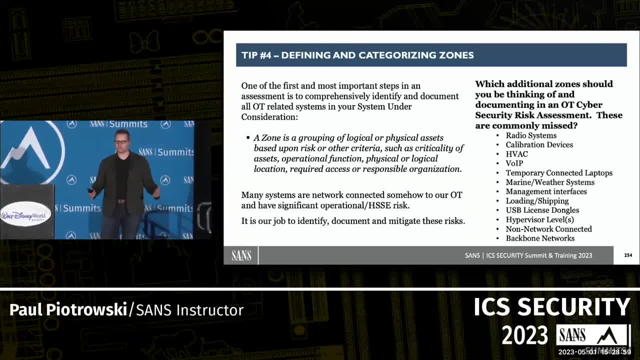 environment. but vendors still have remote access into the HVAC system. that keeps, you know, people safe in the control room. So we identify that under the system under consideration. we evaluate it. sometimes it's just documented that it wasn't under the original system under consideration, but it's our job to look at it right to make sure that. 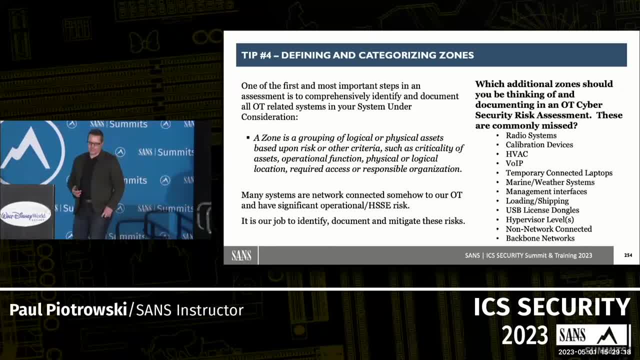 the right controls are being implemented. radio systems also have an hsse impact as well, and then calibration devices are actually unique. so when you go to a good doctor, what's one of the last questions that he usually asks before you leave his office? is there anything else that you'd like? 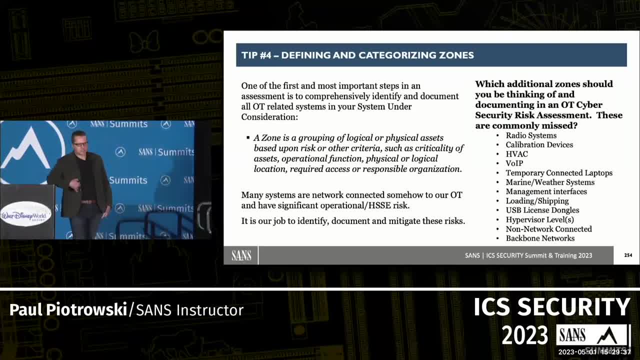 to tell me anything else that you're worried about. so that's one of the questions i've started asking right in my workshops: is there anything else that you're worried about? right, and in my last assessment one of the instrumentation guys said: yeah, actually i do and i'm like well tell. 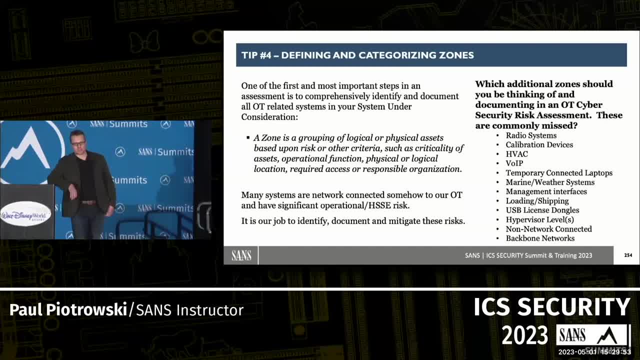 me more and he's like: well, we have these bmex calibration devices and these emerson trex calibration devices- and we actually don't know how many we have- and these calibration devices could be misused by an engineer taking it into the field- you- and reprogramming or recalibrating a safety device in the field, even if the plc is locked. 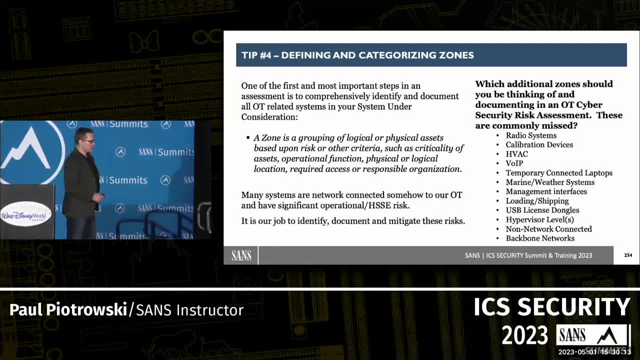 and so like red flags right. you do not want somebody with malicious, nefarious intent or even misuse to go into the field right with one of these calibration devices and recalibrate your sensor without your knowledge, even if your safety system has all um the right controls. so 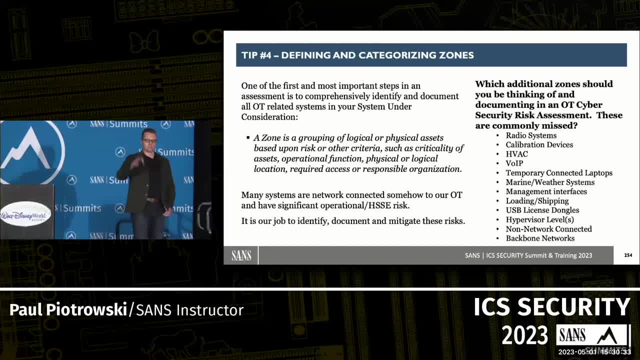 very interesting kind of situation where it came up from the bottom right, you know where you know. it wasn't listed on any network diagram, it wasn't, um you know, identified anywhere. we are talking to the instrumentation guys, talking to the operations guys. what, what else are you worried? 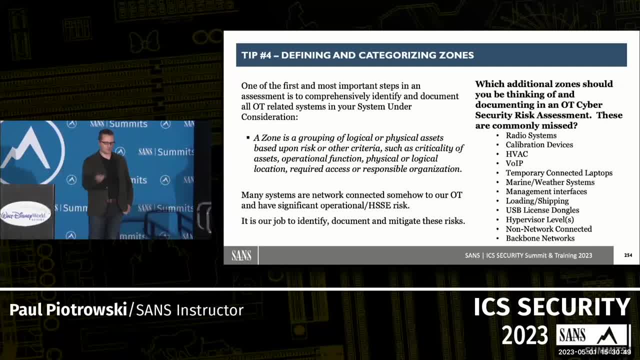 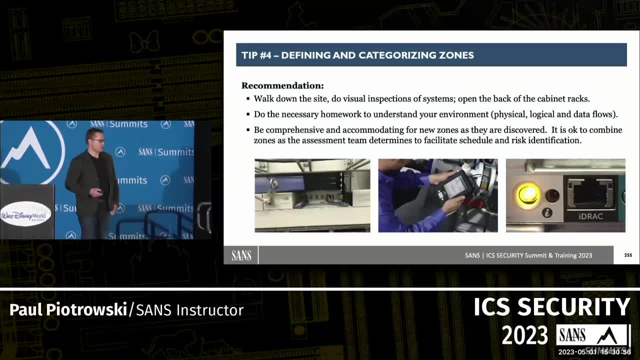 about and the calibration devices came up. i got a picture on the next slide coming up. so um, so many things right that you should be looking at. so usb license dongles right. emerson delta v right. they have a one license key right for the emerson system and one for the hypervisor. 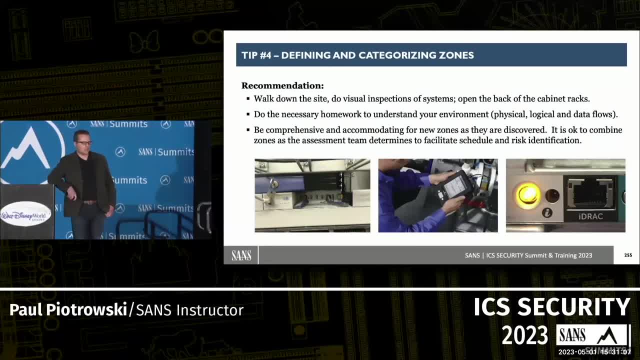 that picture over there has three, because you have a system integrator license as well. so from a physical theft, from a disgruntled employee perspective, you better have some good controls around those usb license dongles, because if those are stolen right, it's a lot of. 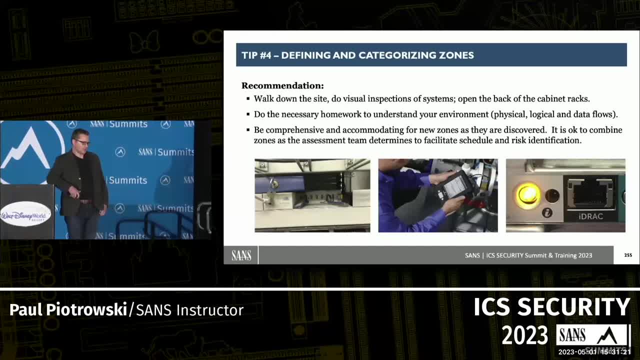 work to re-license, right, your dcs. um, there's kind of workarounds and things like that, but it's going to be a headache for you, right, if somebody you know disgruntled, right, and once that is pulled out, you can't make any changes as well. um, and then there's a picture there of the 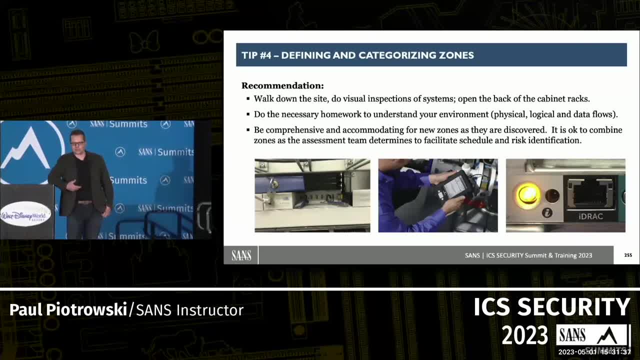 that's the emerson trex calibration device, right, that's a, that's, that's a zone, right, we need to assign, we need to cyber secure that zone. and that could be usually, you know, in that kind of situation, the asset didn't know how many of these calibration devices that they have. so i say well, 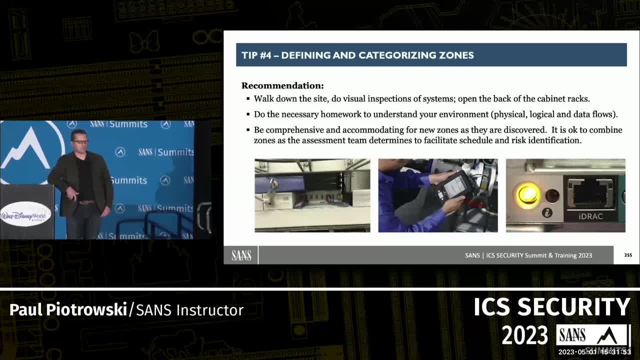 we got to get our hands on it right. we got to start, you know, almost like a retrieval process, um to to scale back on those and, you know, implement some processes with additional training or permit to work or sign out process or whatever it might be right to make sure that. 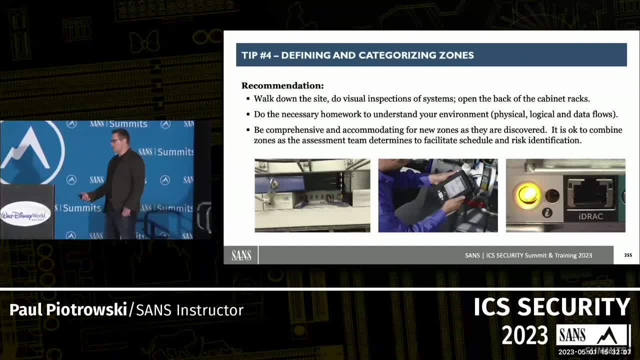 the calibration devices do not get into the wrong hands. um, what about idrac ports? right? there's a lot of remote access actually within the site and rdp is allowed within the idrac and is calvin the password right? so like stuff like that. you know, you don't necessarily kind of focus on it, but I 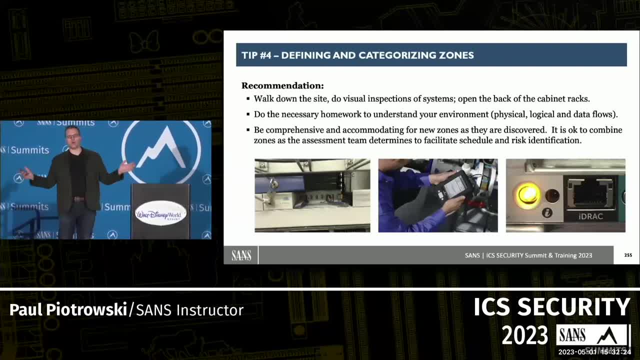 think you know, with a, with a good cyber security risk assessment, you need to kind of open up right and open up kind of pandora's box and kind of look at all these- um, you know, systems that don't show up on a visio diagram. right to be comprehensive in your risk assessment, 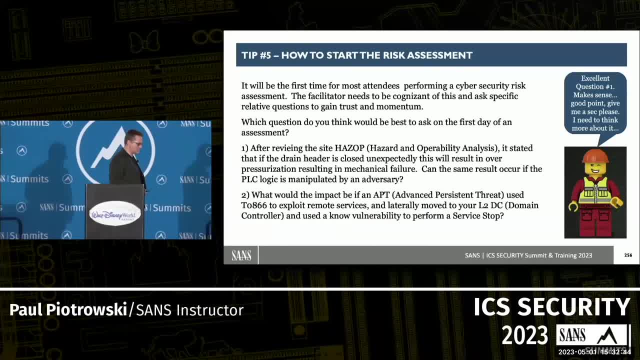 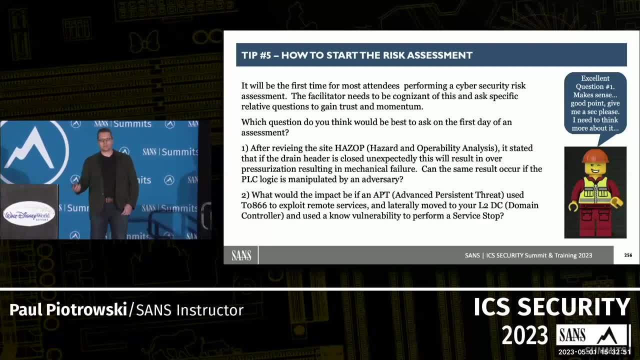 so how do you start the assessment, right? so kind of two, two ways there, right? people in the back will probably have a hard time reading it, so I'll kind of read it, you know. first, one says: after reviewing your hazop, right for your asset, right, it's stated that if the drain header right is, uh is closed. 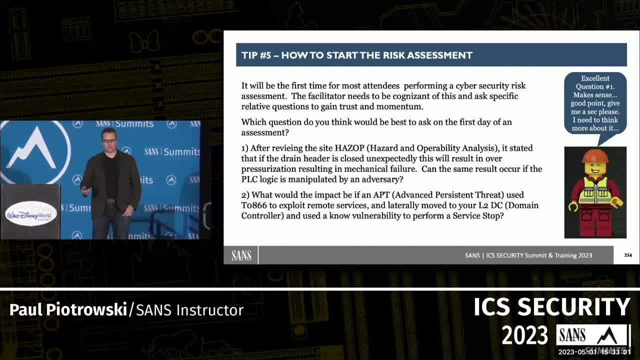 unexpectedly. it's going to create some- uh some- pressurization and mechanical failure right in your piping right. we've looked at it and we think that that could be replicated by changing the data table in the plc. and then the engineers are like, hmm, think about it. they're like we got. 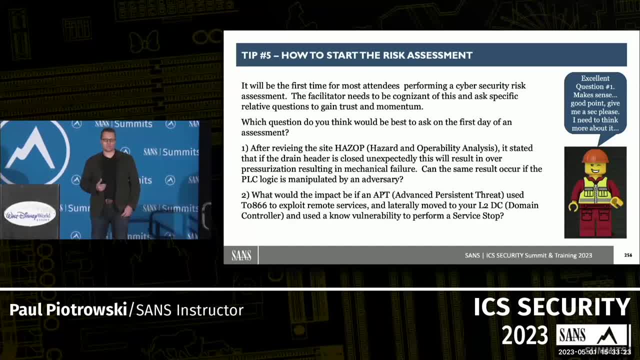 to call Joe right. then they call Joe from the field, then they start bringing in some other guys. then the PID diagrams come out. they're like: yeah, that's actually valid, right, you know that could happen. right, good, catch guys, right. but that's a better way than saying in a zigzag pattern, right. then it'll take four or five months for us to talk to us and then say, okay, you can't go from here without having it. okay, you're pretty good at feet. where it is to ramping up the engage, you went toare and then bubble and net and rolling. right now you're talking about how that works, but it's actually consistent. 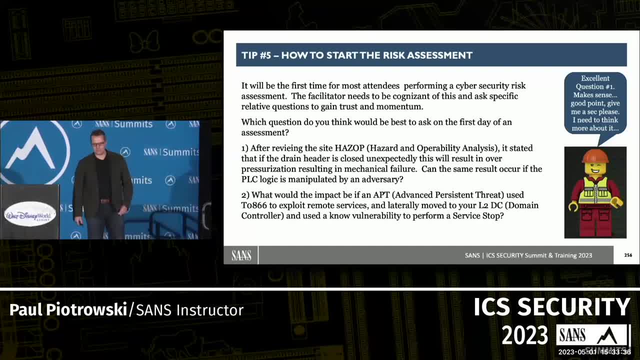 right continue. quite what we're going to talk about. right, we deal with crunch right already, so next step is to also than saying: what if the impact of an apt right using right um remote services, right ttpx right laterally moved from your domain controller, used a zero day, popped your server and did a service. 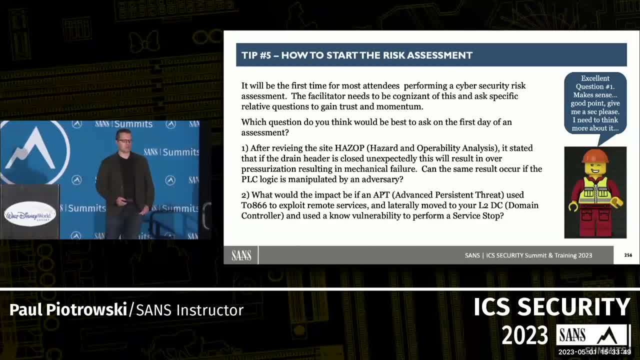 stop right. operations and maintenance ability. who the hell are you? right, go back, right. you're you're, you're out of touch. right, so use the has op right to build trust with your operations and your maintenance teams. right to say that cyber is important, that plc right could be modified and 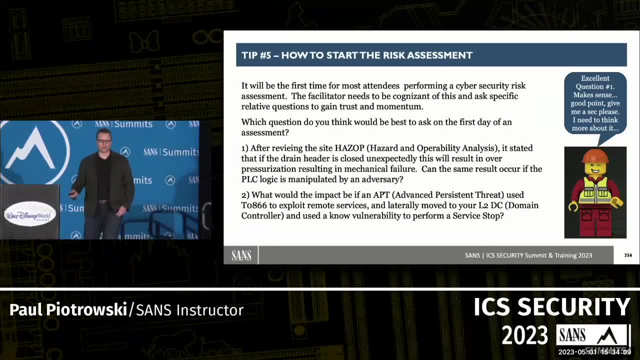 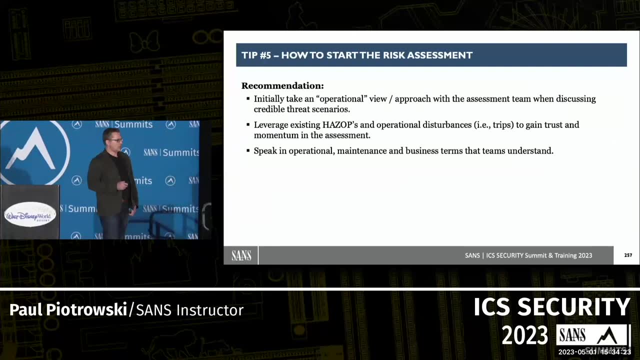 what you've identified in the has op right could be cyber hackable, and then you'll get their trust, they'll perk up, they'll start bringing in their additional diagrams and the the whole engagement will be much more fruitful for you. so, uh, recommendation: initially take an operational view. 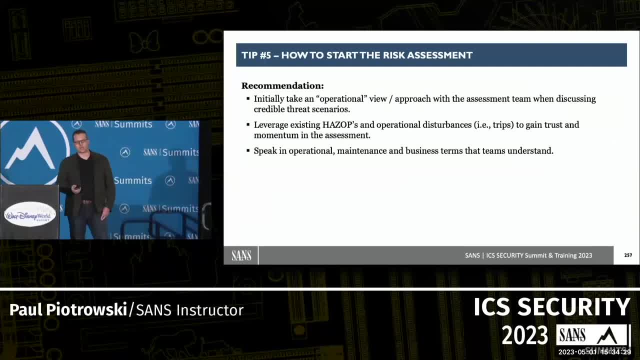 right, leverage right, the, the has op right. use their language right, don't come in their guns blazing right with you know, with cyber lingo and and uh, you know all the, all the threat, all the threat names that we have and all the um, all the various cyber kind of related uh terms that we use in our day-to-day. they don't. 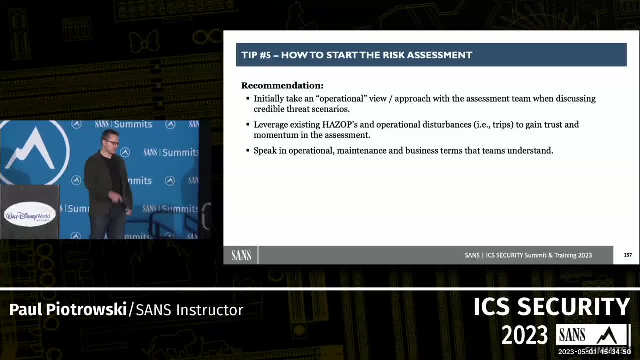 understand it and they don't respect those very well, but they respect somebody who can talk about the mechanics, right, and the process and that can understand the has op, or at least just trying to understand the has op. you will get way more progress right doing that. um also ask, right you know it's a dialogue, right? what additional trips have you had? 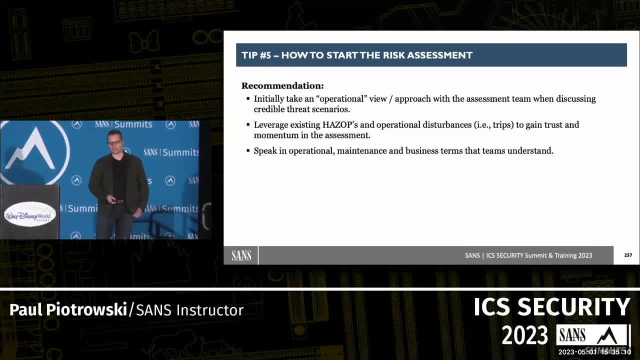 in your plan, right, what upsets have you had right in your facility? right, can you give me a report and then say- and then kind of go through that with a fine-tooth comb- um, to say could it, could it have occurred, right, uh, with with cyber means, right, and uh, that would. that will get you very far. 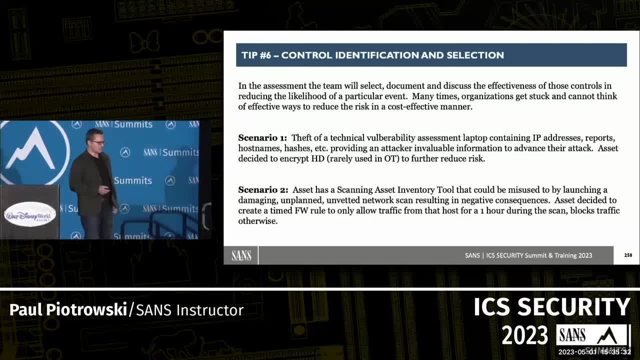 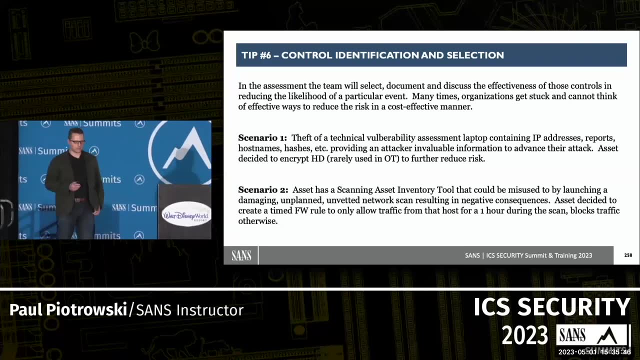 so control, identification and selection right, this is a big one too. um, we as cyber security professionals, we like technology, we like tools, we like to buy licenses, all those kinds of things, but sometimes it's the simple controls that are the most effective and the best right for an asset. 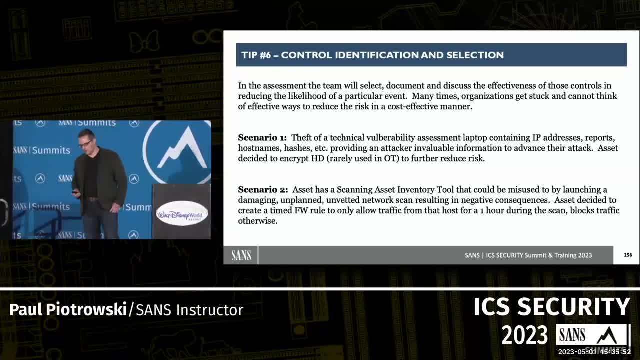 and so some examples there: right, there's technical transient cyber assets. right, if you're kind of a nerd guy, theft of a technical um. so one asset had a tech, a technical vulnerability assessment uh tool, uh that they use to scan and do va in their network, that they kind of moved around the asset all the time. and uh, that laptop had uh pen test. 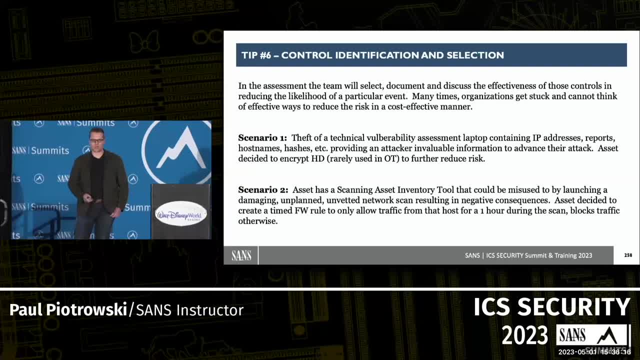 reports had ip addresses, a whole bunch of intellectual property that would be ideal for an attacker to have right vulnerabilities that were found on the network. you know ranges, you know host names, you know you name it. it was all located on this laptop. so we started talking about: well, how do you secure that laptop? well, we only have one of them. it's locked up in this room. 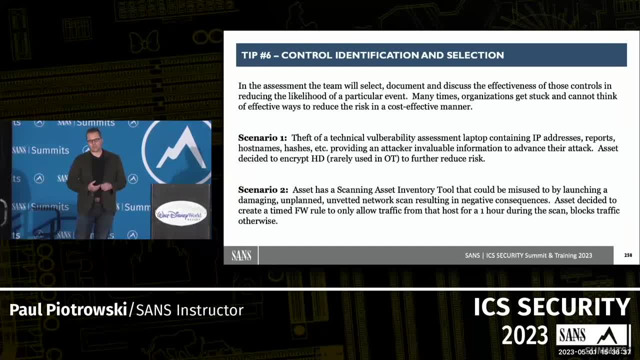 et cetera, et cetera. and, uh, we actually said, well, i think we can do a little. and then i started: well, what else could we do? and they're like: oh, don't worry about it because it's fully encrypted, right, so we encrypt it. you know data at rest. so even if it does, you know, grow legs and walk away. 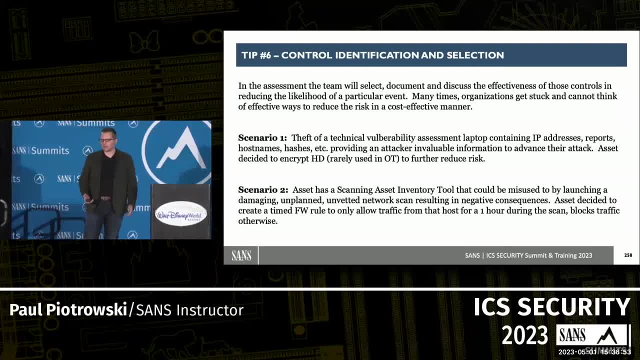 um, nobody's going to be able to- uh to access it, right? all that data is encrypted on the hard drive. so i thought that was actually quite cool, because normally we don't use a lot of encryption in our ot networks, but this asset decided to encrypt the hard drive to protect the intellectual property of their va tool. so i thought that. 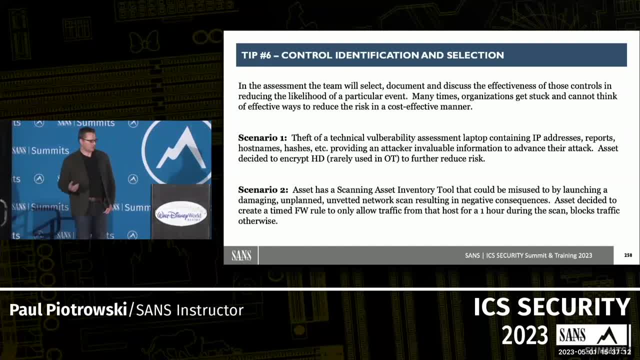 was kind of neat, very simple, right um. another example: an asset had a windows xp machine. they virtualized it. so that was kind of cool and i started asking: right, it was an engineering workstation, that was windows xp. and they started doing the risk. obviously an engineering workstation. 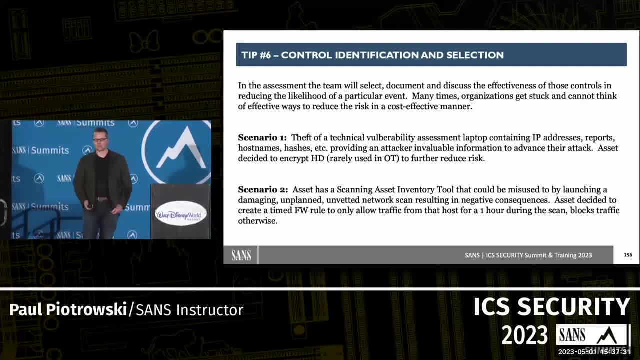 and they said: look, you know, we've got a lot of privileges right. there's usually project files on it. you know, it is something that attackers would love to get their hands on. and the site said: don't worry about it, we shut down the vm. we only use right the windows xp machine once a year. 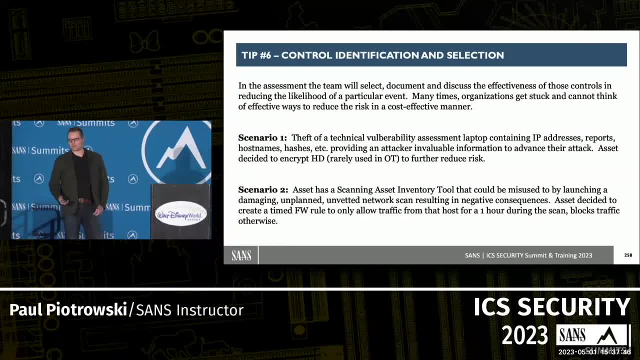 right, so we shut it down. we have no use for it, so we shut it down. and then i said, oh, that's pretty cool. and then they said, to boot, we also have a pm preventative maintenance activity. every quarter we spin up the engineering workstation just to make sure that works. so i thought that was quite 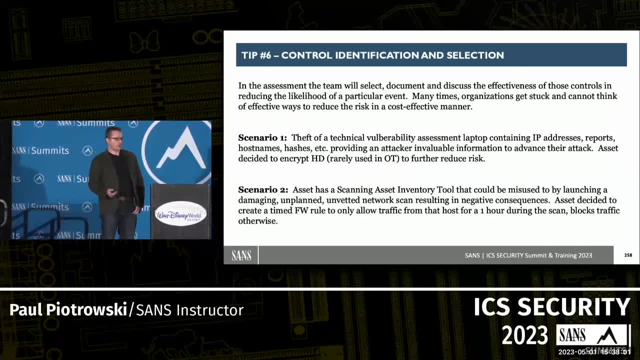 so that was kind of cool. um and then another example: one asset had on the network. they had a scanning tool on their network that they periodically do asset scans right in different network segments and they were very uh, the site was very mature. they actually implemented a timed. 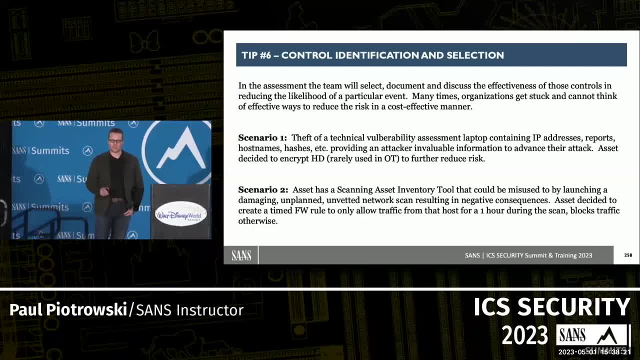 firewall rule. right, so you can. on firewall rule, you can say that this firewall rule only applies for a one hour, you know two hour duration while the scans are being accessed. so i thought that was really cool, where they went the extra distance to say: we know that this. 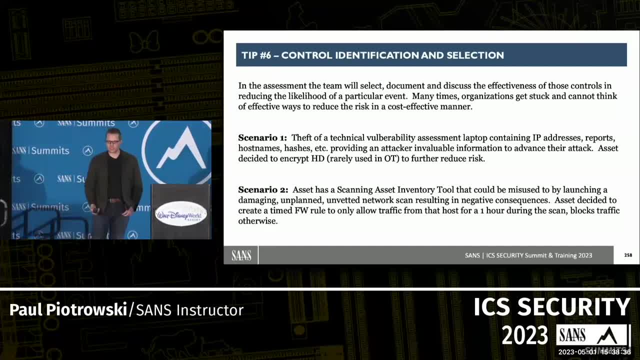 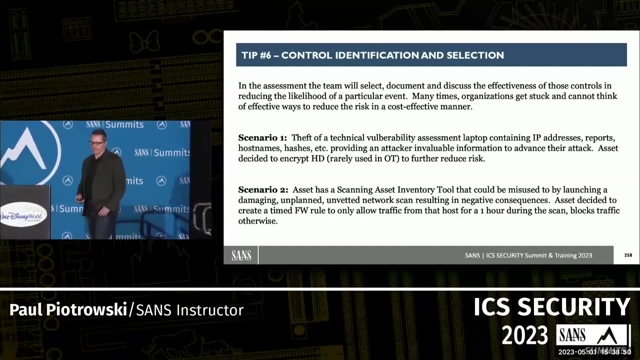 machine is highly vulnerable. right, it could be used as a pivot point for an attacker, but we're mitigating that by implementing a firewall rule that's timed only for the duration of the scan and then that, and then the firewall rule resets and uh blocks the traffic. so i thought that was. 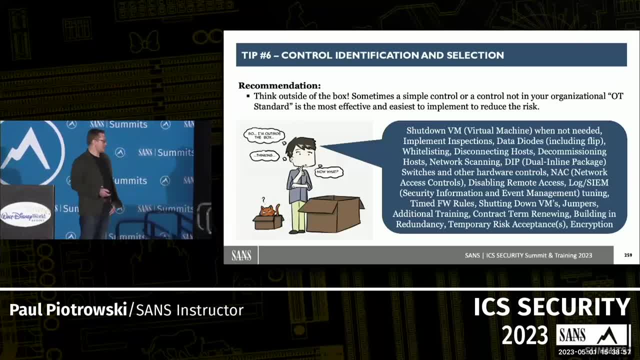 really cool. so a little busy slide here right. but i think you know it's really important to understand that there is certainly some opportunities out there with the environment and um, you know we need to. as cyber security professionals, we need to have a toolbox and we have to have the right tools for the right job and implementing. you know whitelisting knack. 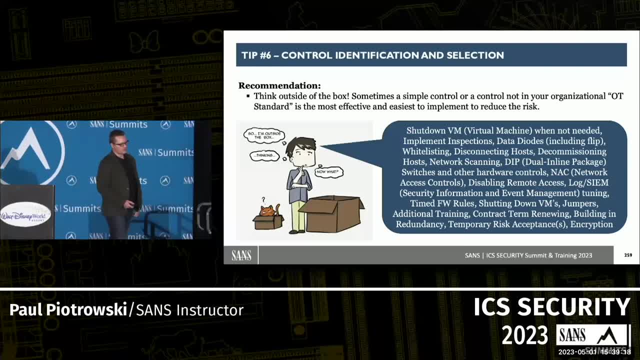 all this kind of stuff, you know, um, yes, it might work in some places, right, or might be the right control, but maybe shutting off or decommissioning, getting rid of the of the of the machine, um and the attack surface, is a better option, right? so think outside the box a little bit. um in uh. 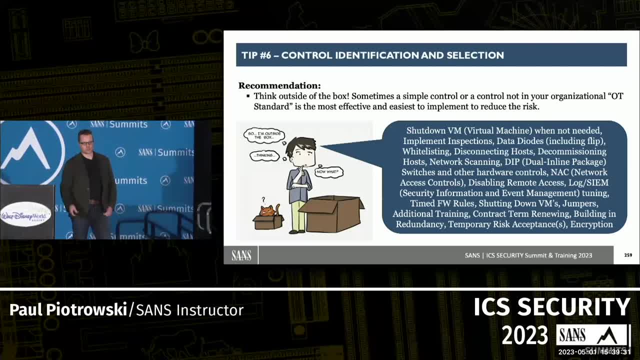 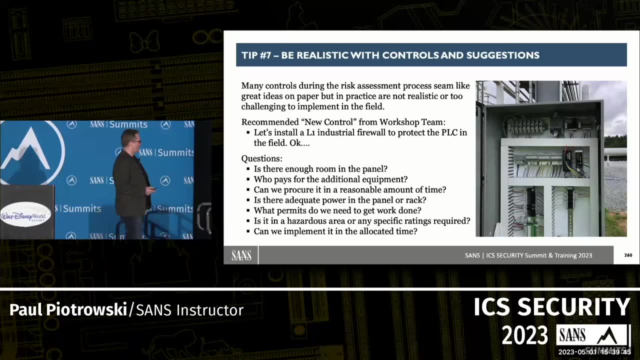 in doing your cybersecurity risk assessments. It's not all about buying additional tools and additional product or licenses. Sometimes it's the simple things that are the most effective. So last tip here: be realistic with the controls that you implement. So if you're somewhere in head office and you're doing a cybersecurity risk assessment, 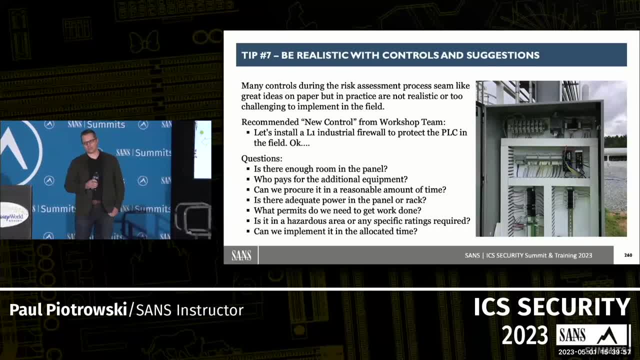 it's very easy to say, oh, we should implement an industrial firewall in this location, we should do this, we should do that. Once that recommendation is put into place, you're going to get some pushback. Is there even enough time to actually make that change? 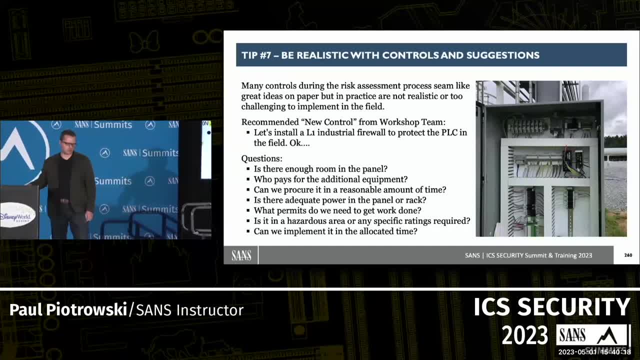 Who's going to pay for the additional hardware? I've seen situations where you make that recommendation and they say, well, you made the recommendation, give us budget. Well, it's your asset, you need to do it. No, we have no budget, And so you get into those interesting. 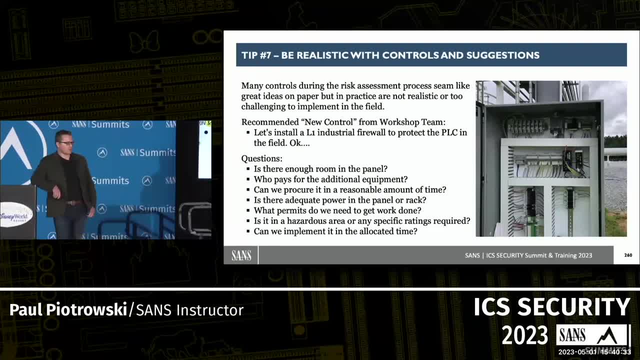 challenging discussions on who's actually going to pay for the equipment or for the additional cybersecurity controls that you're recommending, And, with supply chain, it makes it very difficult nowadays as well to get equipment. So you got to think, yes, okay, we're implementing or we want to implement this, but can we even get it in the right of? 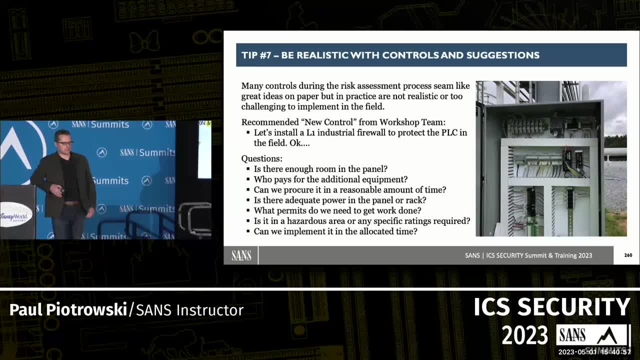 time? Can we implement it? Can it get across the borders? Can it even fit in the rack, in the panel, in the field? Do we have adequate power for it? et cetera, et cetera. This is where operations maintenance have to come in and say, yeah, we actually have. 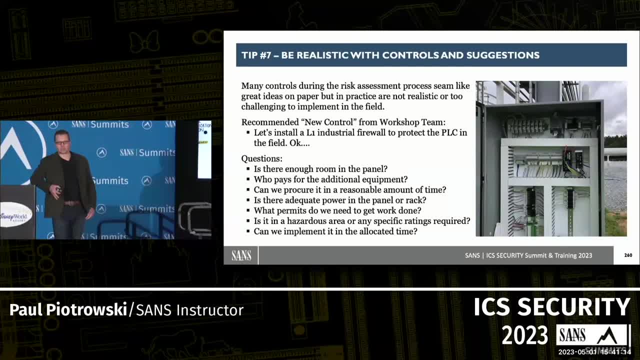 room in the dinner rail and we have power. We have to check with electrical, but I think we have enough power in that rack, in that panel, to implement that firewall. So how do you get it in the right of time? How do you get it in the right of time? So how do you get it in the right of time? You have to think about what you're going to implement, but you also have to think about how you're going to implement it, And you're going to have to make sure that you're going to implement it, And so 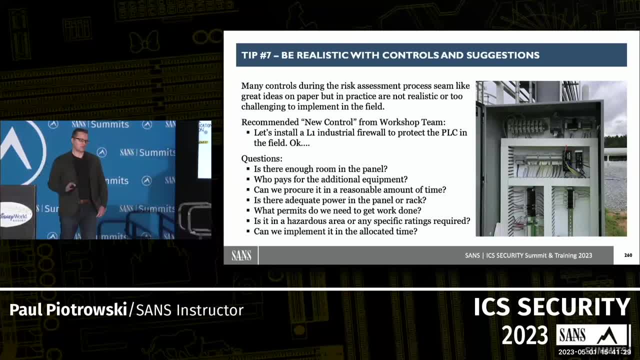 we are going to learn from you, but you also have to think about how you're going to implement it. So those are the two things. So you want to be very cognizant that in head office or in a nice conference room. 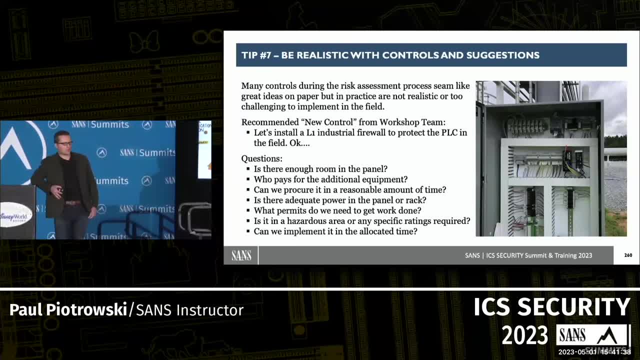 it might seem like a good idea. but then who's going to pay for it, who's going to operate it and who's going to maintain it? You do not want your solutions to die on the vine because there's no ownership and no buy-in from the asset level, from the controls. 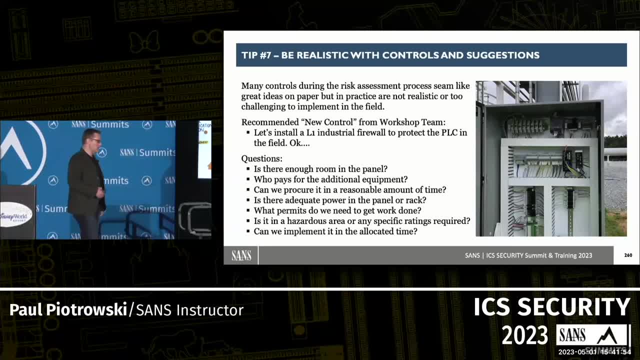 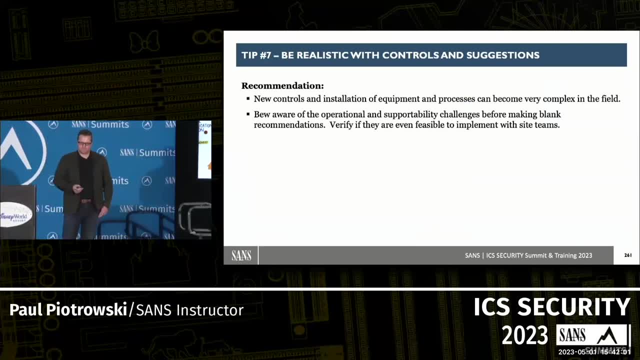 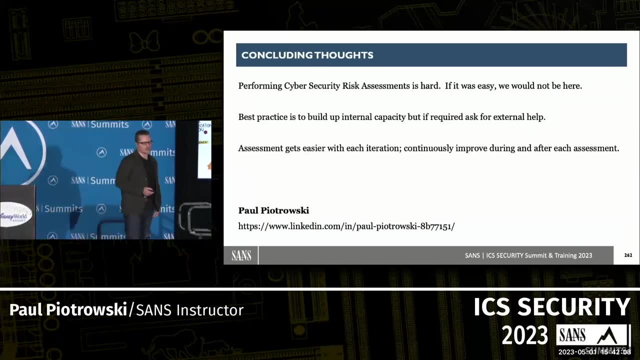 make sure whatever recommendations you're doing are very are sustainable right in your organization. yeah so, concluding thoughts right, um, risk assessments right, are hard, right. if, uh, if they were easy, we wouldn't be here right, there wouldn't, there wouldn't be a conference like this that is put on by rob and rob and tim. so you have to build that organizational muscle. 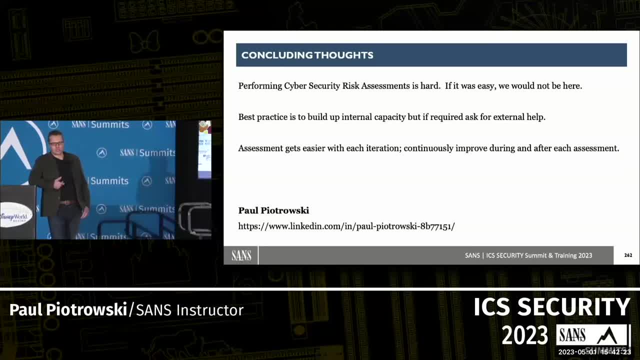 right, i'm a big proponent of building capabilities in in-house. but sometimes you do have to call and pick up the red phone and ask for help, right, so you do want that help. sometimes. right to get that mentoring, to get framework, to get the training, but make sure that you have skin in the game. 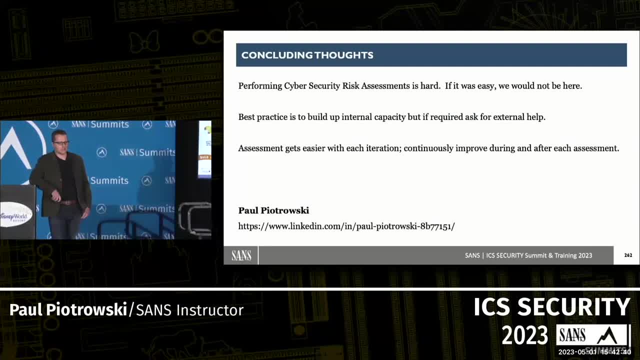 and that you actually invest and and and learn the process and then try to build that organizational muscle in your organization, because there's going to be more of these required and i think, as a community, i think the whole theme right of this whole conference is, you know, building the 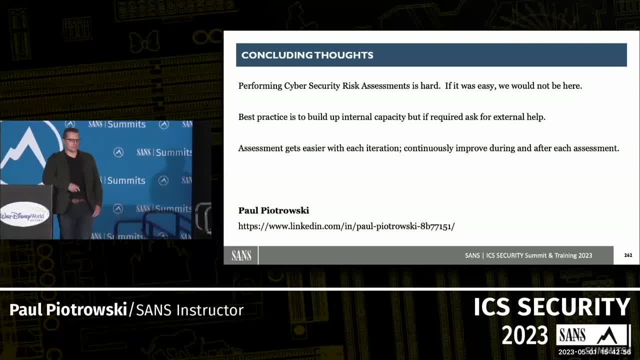 community, you know, doing info shares and knowledge shares, etc. i think as a community we need to get better right at identifying and identifying the risk, identifying good controls, prioritizing controls, and uh and operating them, and and uh and make and communicating it, you know, to our leadership. so assessments do the first assessment that you do. it's not going to be perfect, right.